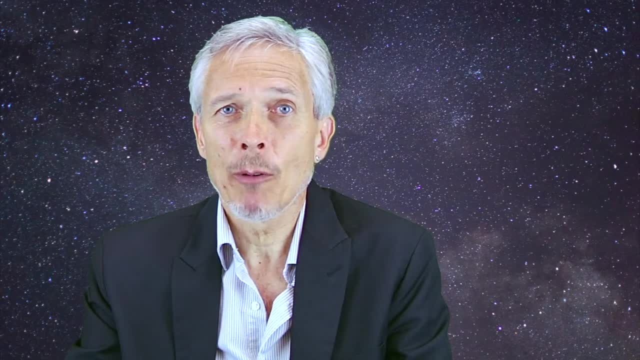 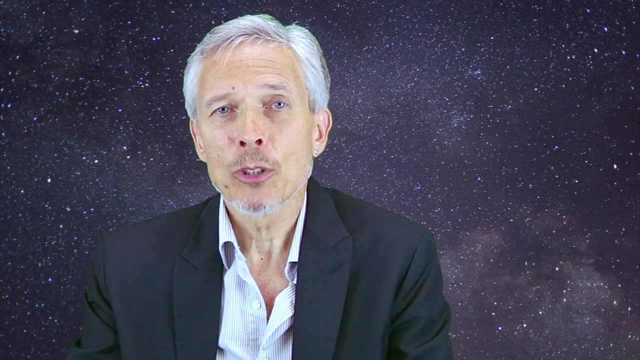 We've seen that something extraordinary lurks at the heart of the Milky Way galaxy: a supermassive black hole, 4 million times the mass of the Sun. But even before this object was discovered, it was understood that some external galaxies have strange things going on in their nuclei. 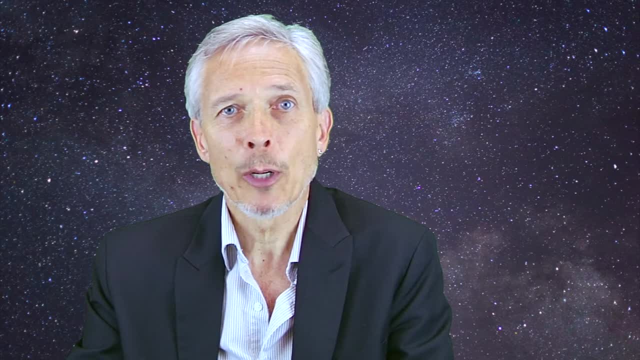 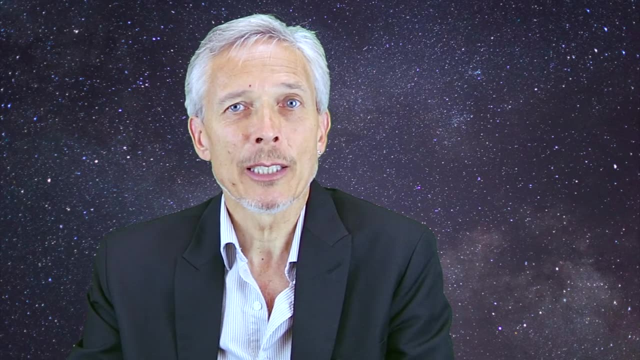 and often they were variable in their luminosity, variable on timescales of weeks. There's a simple argument based on light travel time that says that if any coherent object is varying on a particular timescale, it must be smaller than the distance light could travel in that timescale. 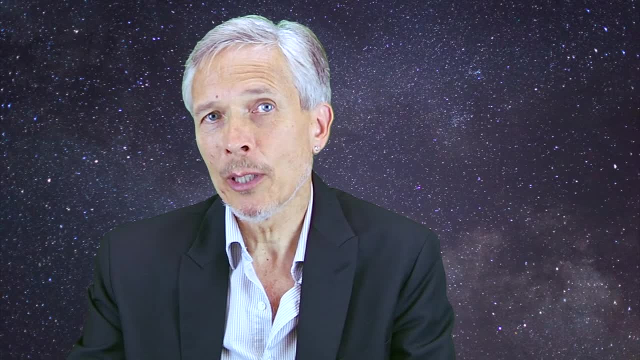 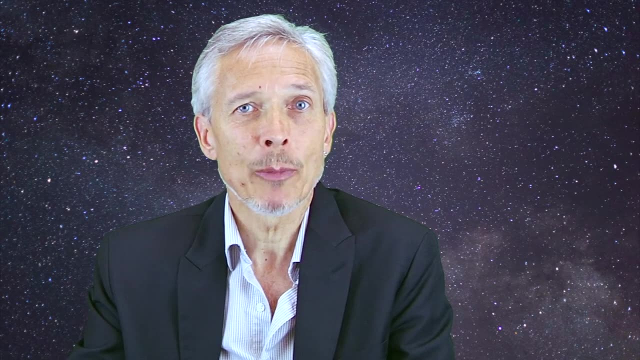 So the Seifert galaxies, whose light output from the nucleus was varying on timescales of weeks, must be smaller than light weeks across and have an enormous amount of radiation coming from that region. Seifert also took spectra of these galaxies and showed that their centers had broad emission lines. 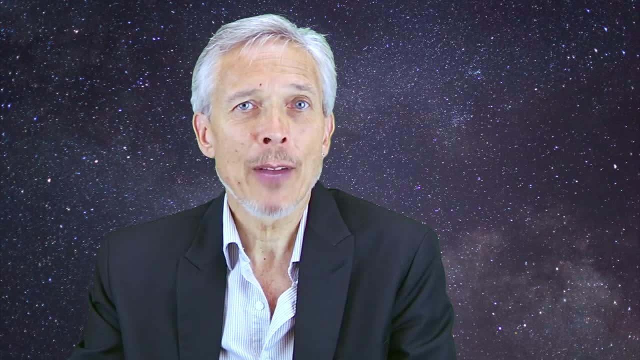 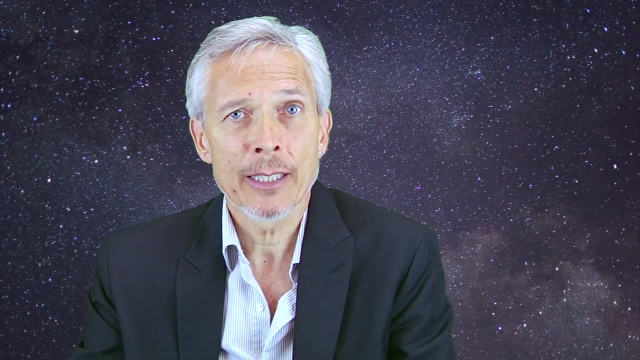 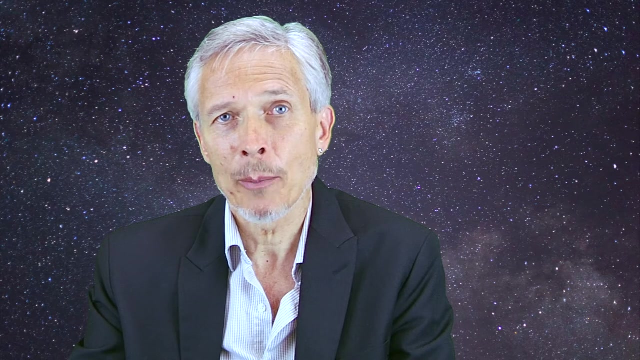 The breadth of an emission line is a Doppler measure of how fast the gas was moving. Unlike the gas in orbit around the Milky Way disk, which has velocities of only a few hundred kilometers per second, the gas in the center of these galaxies was moving at speeds of thousands of kilometers per second, up to 10,000 kilometers per second. 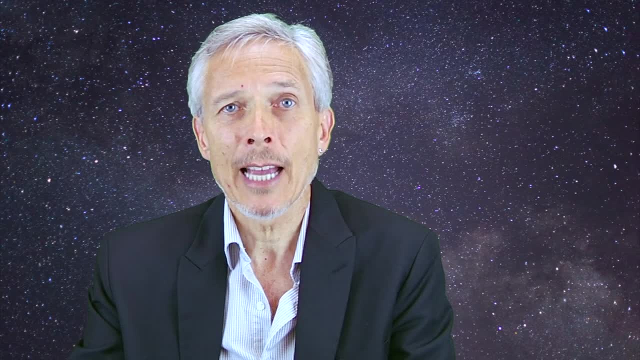 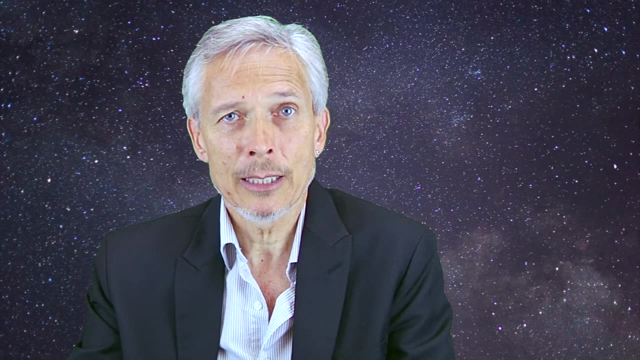 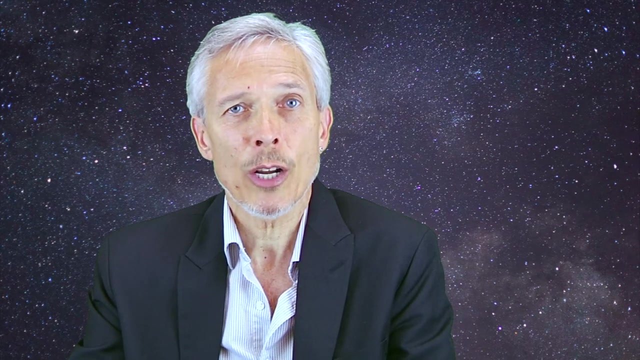 Something very exotic must have been driving these high gas speeds. Next, as infrared techniques were perfected in the 1970s, people noticed that the Seifert galaxies also had intense infrared nuclei. Essentially, they had large amounts of electromagnetic radiation coming across the spectrum. 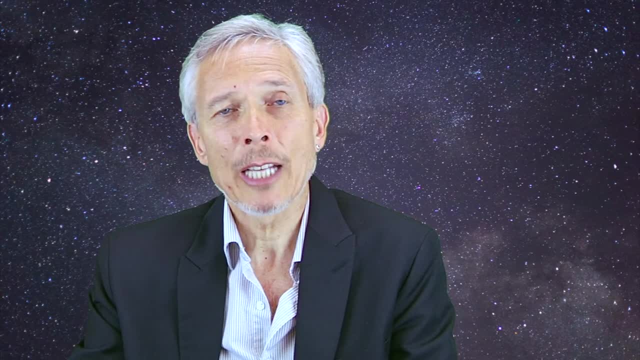 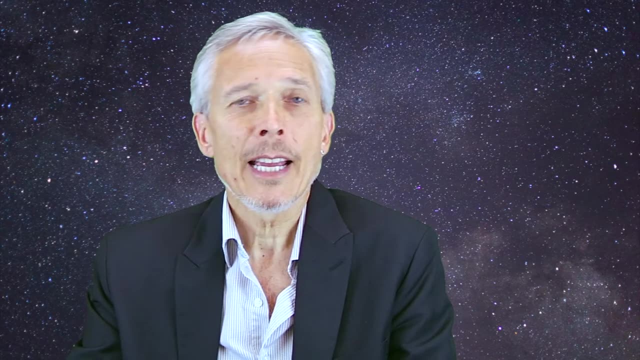 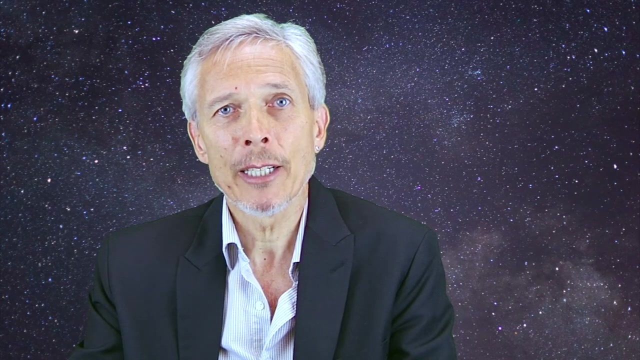 In extreme cases, the luminosity of a Seifert galaxy nucleus could vary by more than the entire light output of the Milky Way on timescales of a few weeks, A decade or so. after Seifert, radio astronomy came out of its infancy and started to measure populations of radio sources in the sky. 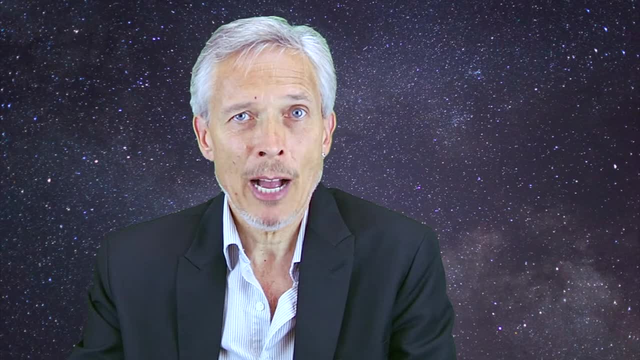 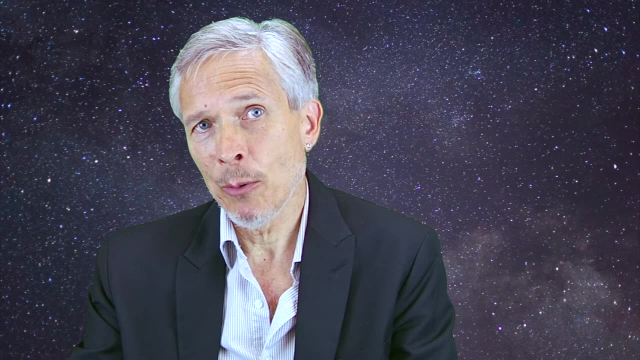 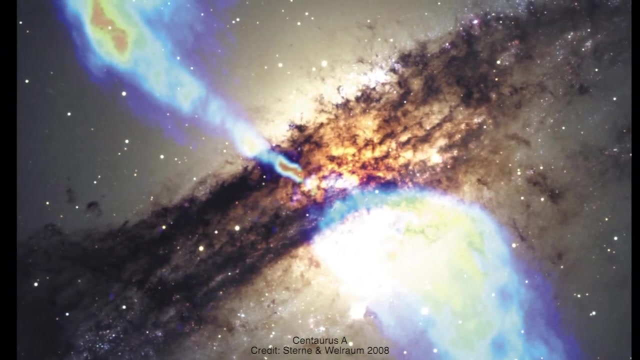 The brightest of these radio sources were phenomenal in their radio output, far exceeding the radio emission from our own galaxy. As radio astronomers developed the technique to map out the radio emission as opposed to just detect its intensity, they noticed that the radio emission often was not coming from the center or the nucleus. 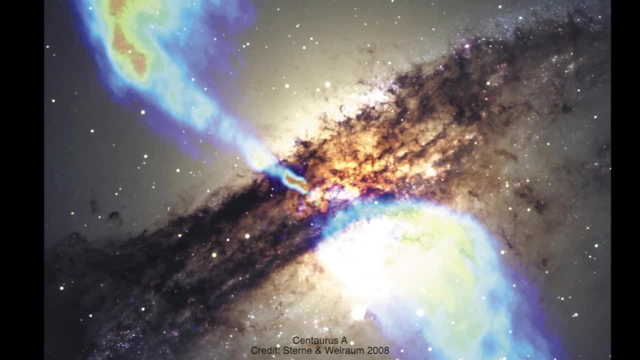 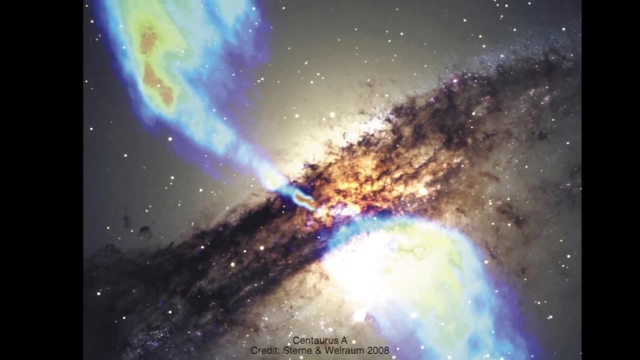 Sometimes it was coming from twin lobes of plasma at distances of up to a million light years. Something was putting energy out and making it travel over these vast distances into intergalactic space. The mechanism for this radio emission was supposed to be synchrotron emission. 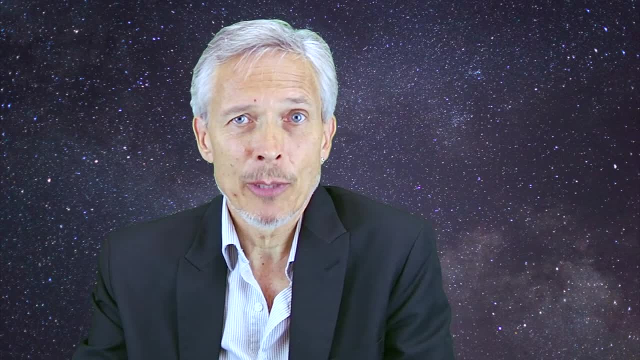 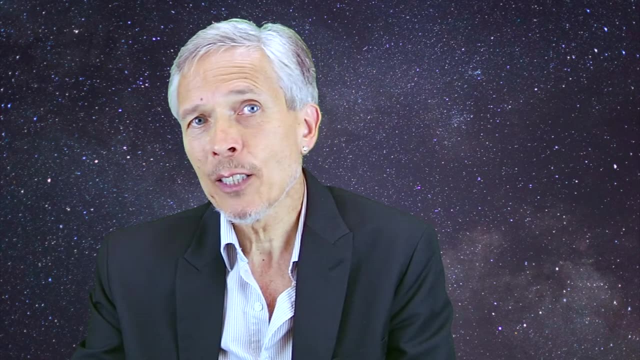 The key diagnostic to indicate that it was synchrotron emission was the fact that the radiation is polarized, which means the particles are being accelerated in a coherent magnetic field. As this information accumulated in the 1950s and 1960s, 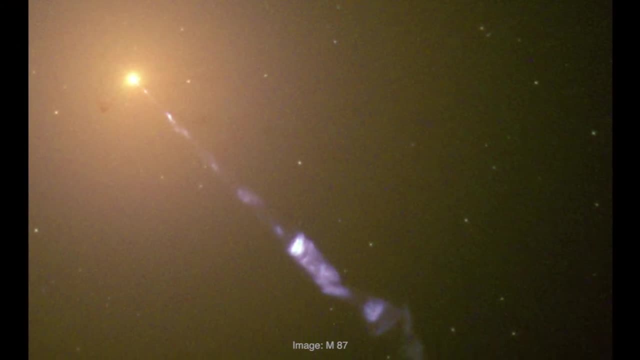 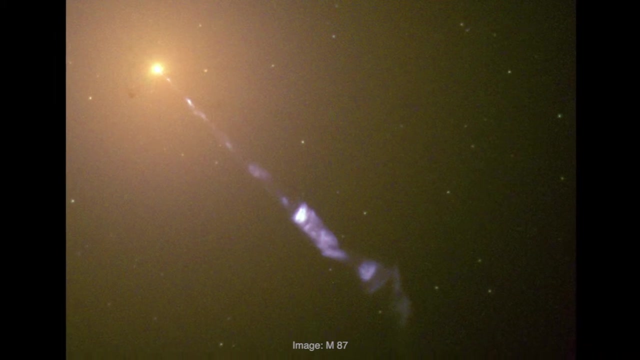 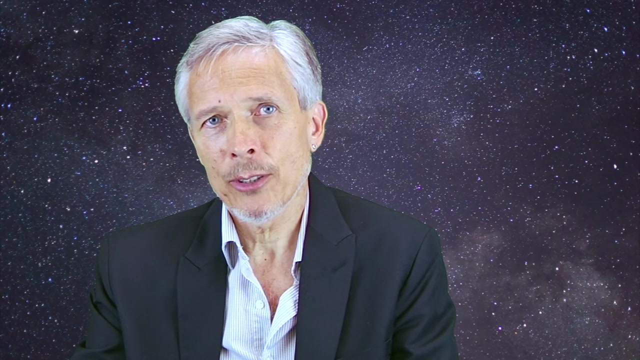 people realized that the nuclei of many galaxies had extraordinarily energetic phenomena occurring. Essentially, plasma is somehow being ejected from these galaxies at speeds close to the speed of light energies far beyond the reach of terrestrial accelerators. To drill down into the center of these external galaxies takes very high angular resolution. 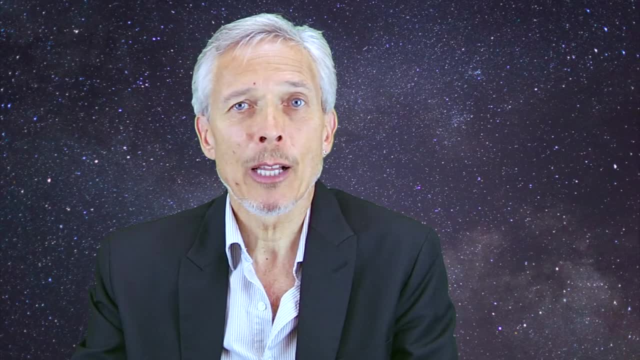 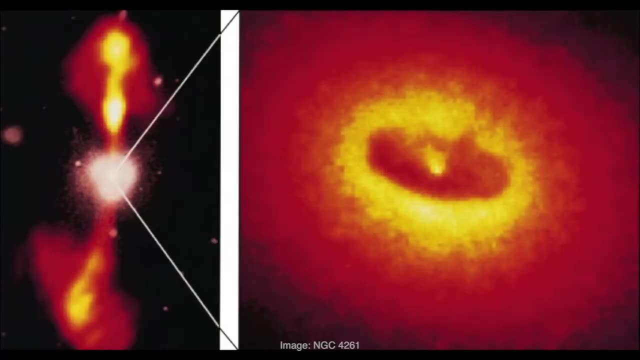 That resolution came to radio astronomy through the development of the interferometric technique. In optical astronomy it came with the launch of the Hubble Space Telescope. Eventually a hypothesis emerged to explain these phenomena By analogy with the argument for the center of our own galaxy. 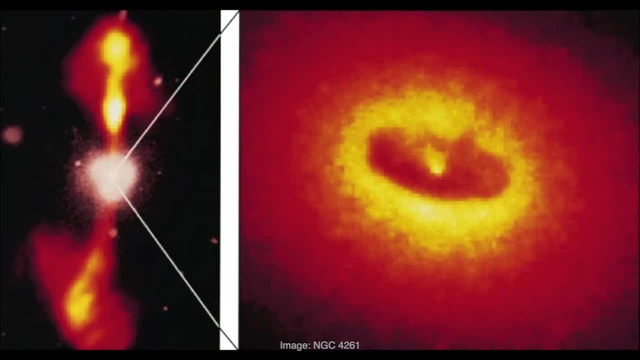 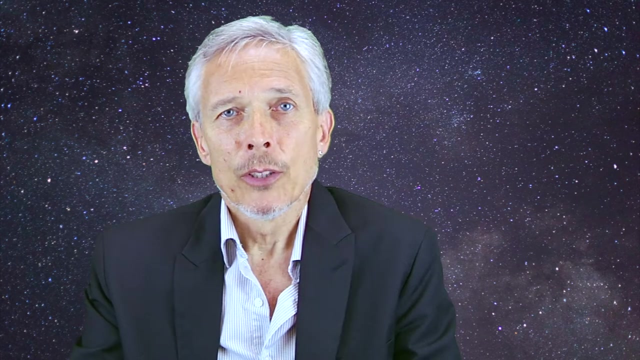 it was quickly realized that a hugely dense star cluster could not possibly explain these various phenomena, especially the radiation at non-visible wavelengths like radio waves and x-rays. The hypothesis that emerged was of a gravitational engine, a supermassive black hole. The supermassive black hole is at the exact gravitational center of a galaxy. 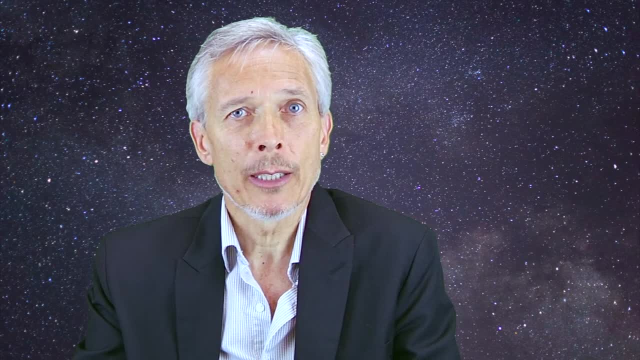 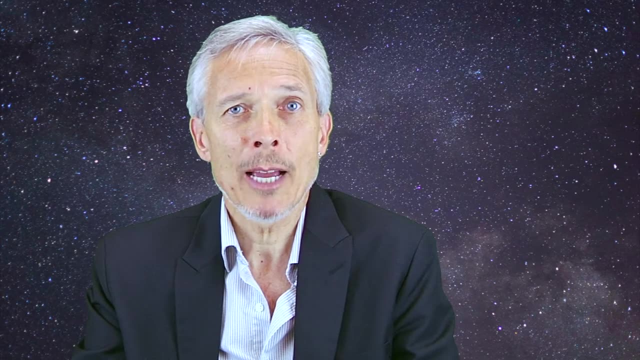 It's the gravity pit into which matter is falling, and therefore the black hole is presumed to have grown over time to reach the sizes currently seen in the universe, up to billions of times the mass of the Sun. As matter fell into the black hole, it was accelerated. 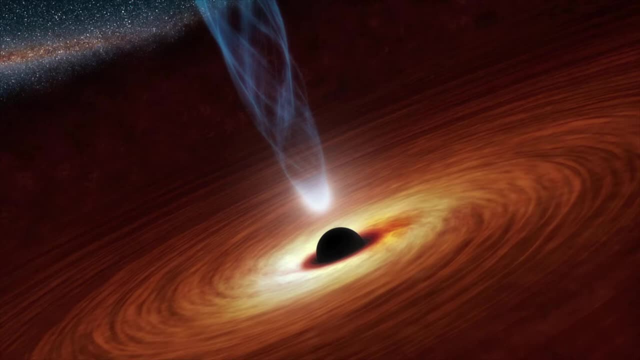 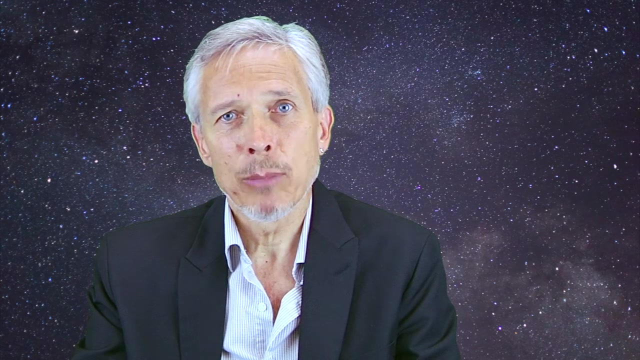 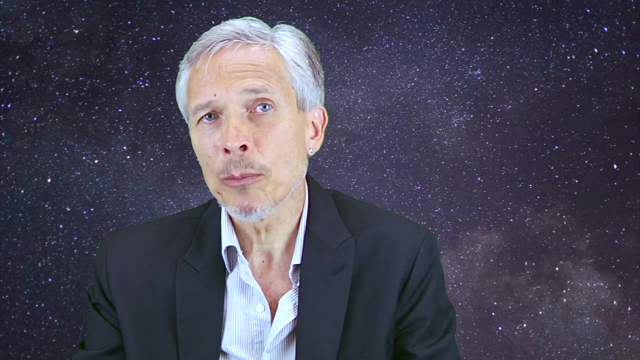 and the accelerating particles produced enormous amounts of electromagnetic radiation across the entire spectrum range of billions in wavelengths. Although a black hole is indeed black, as matter goes into its death spiral near the event horizon, it can release enormous amounts of energy. In principle and in the theory. the efficiency of a gravitational engine can be quite high: 10 or 20% of the mass energy released. Remember that normal stellar fusion releases less than 1% of mc2 of the mass energy. so this is 10 or 20 times more efficient than stellar fusion. 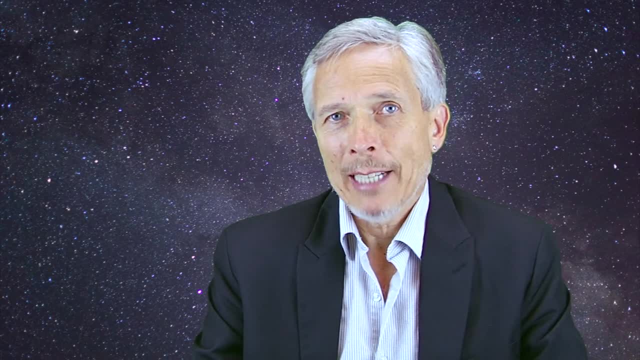 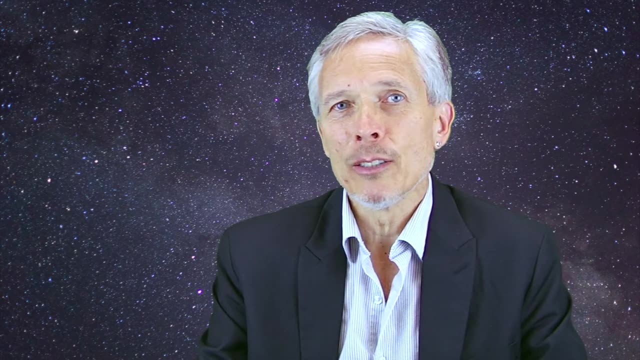 By the early 1960s a zoo of active galaxies had been discovered, starting with the galaxies that Carl Seifert found in the 1940s, spiral galaxies with bright, luminous, variable nuclei, adding to that in the 1950s. 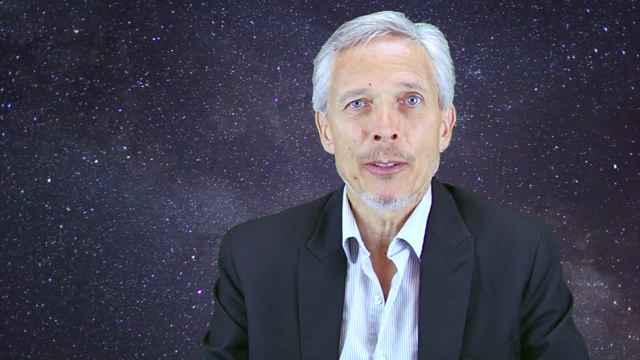 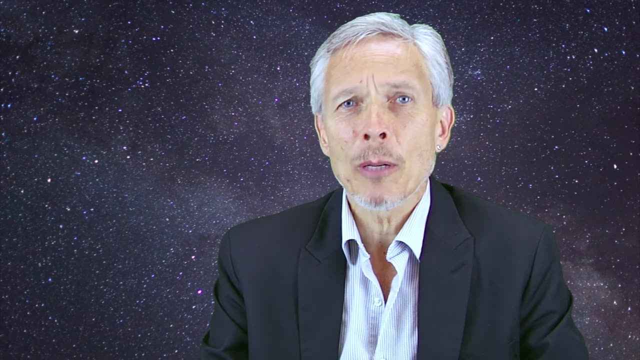 radio galaxies found with plasma ejected far beyond the realm of the galaxy itself, and then, through those decades, an increasing number of interacting or merging galaxies where something extraordinary seemed to be happening in the combined nucleus. Clearly, interactions was fueling activity in the nucleus. 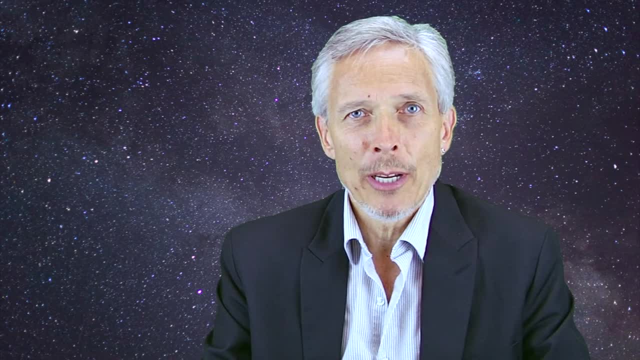 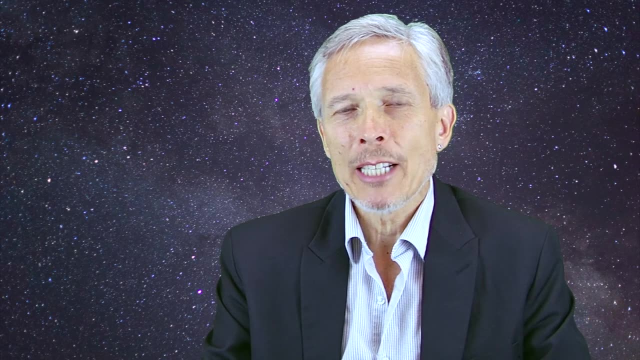 In the early 1960s, a young researcher called Martin Schmidt, from Holland but working at Caltech, took data with a 200-inch telescope at Mount Palomar. He took spectra of bright star-like objects that seemed to be associated with it. 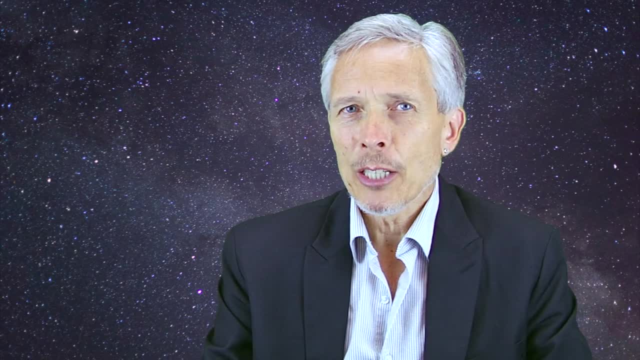 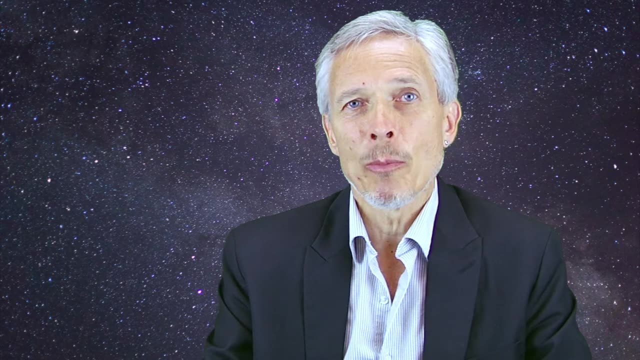 particularly with strong radio sources. from the Cambridge surveys It was unusual to find a star-like object associated with a radio source. The Sun and other normal stars have very weak radio emission, so what possible star could emit such intense radio waves? Well, it turned out they weren't stars at all. 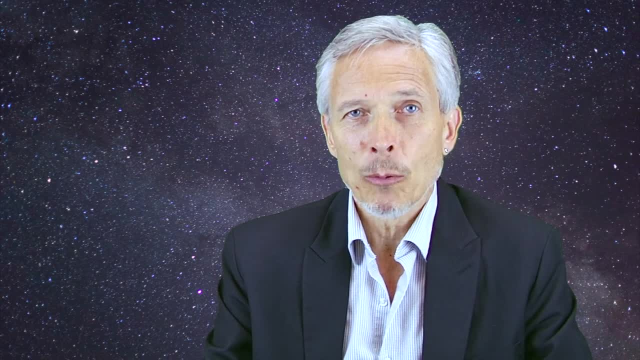 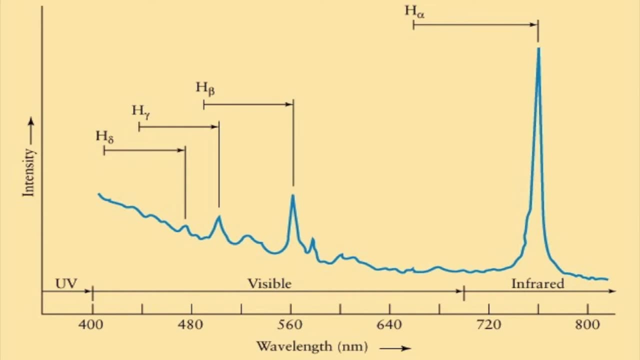 They were nearly star-like objects, quasi-stellar objects that were actually at phenomenal distances from the Milky Way. Martin Schmidt solved this puzzle by noticing that the spectral features were those of normal elements like hydrogen and helium, but shifted to the red by extraordinary 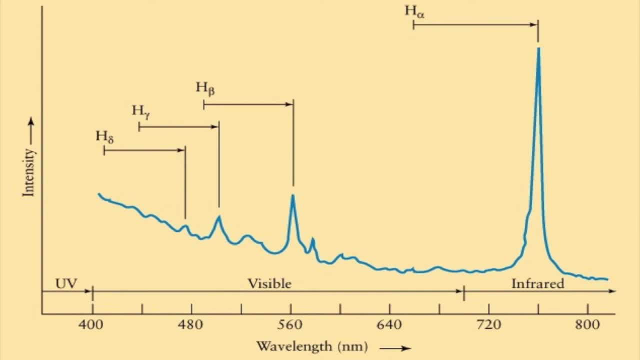 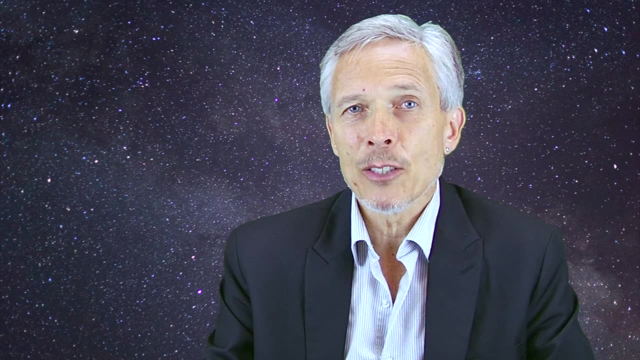 unprecedented amounts- 10,, 15, 20%- in the spectrum. By noticing this, Schmidt made an amazing discovery. He discovered that there were compact galaxies at distances of billions of light-years from the Earth that were emitting as much radiation as a thousand galaxies. 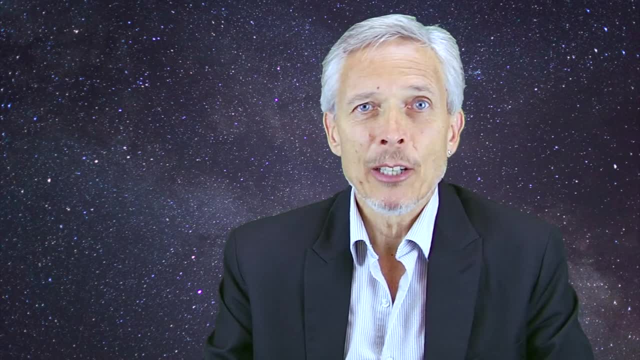 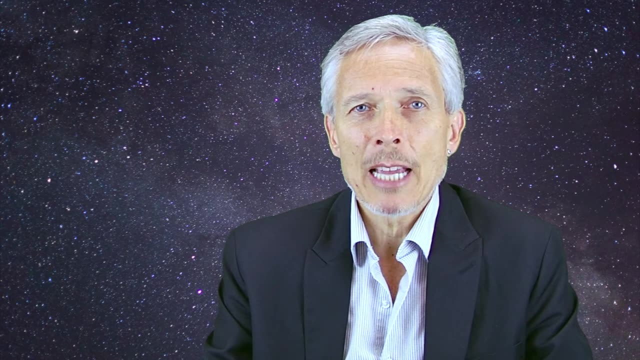 These objects- quasars- were marked by intense radio emission, by very broad spectral lines indicating gas in the nucleus moving at nearly relativistic speeds, and by a very strong ultraviolet emission beyond that expected from any stars. Clearly this had to be non-thermal emission. 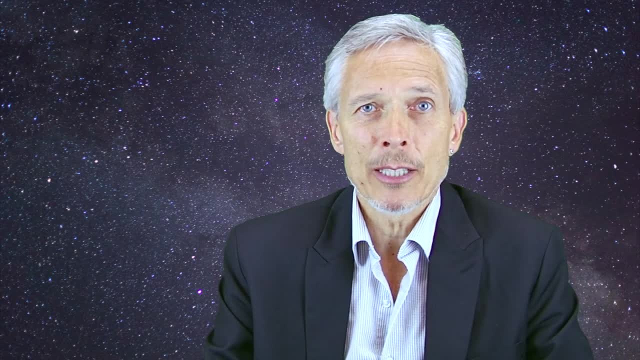 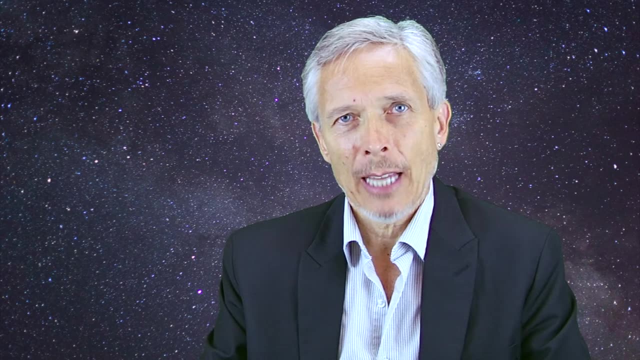 something related to the synchrotron emission that gave rise to the radio activity. The first quasars were intense radio sources and they were typically numbered by the 3C catalog or the Third Cambridge Radio Catalog. 3C48 and 3C273 were the first two quasars discovered. 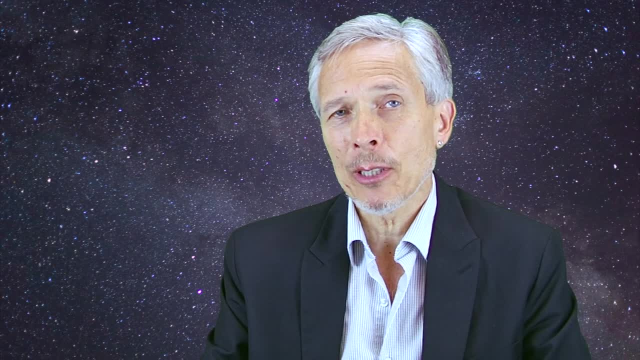 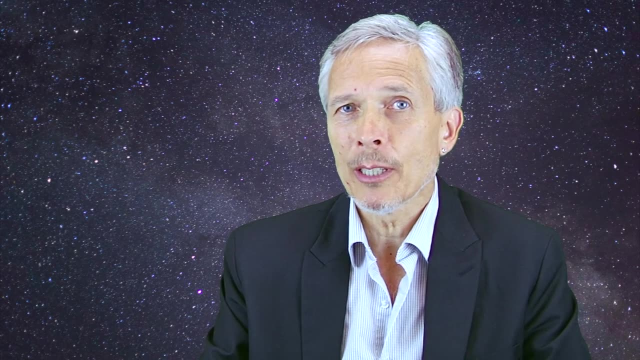 And while the compact radio emission was the tell-tale that led optical astronomers to the optical counterpart, it soon turned out that most quasars did not have strong radio emission. Non-thermal optical and ultraviolet emission could be present with no strong radio waves. The number of quasars grew by leaps and bounds in the 60s and 70s, until catalogs contained thousands of them and their distances approached 5 to 10 billion light-years from Earth. It's hard to visualize a quasar. 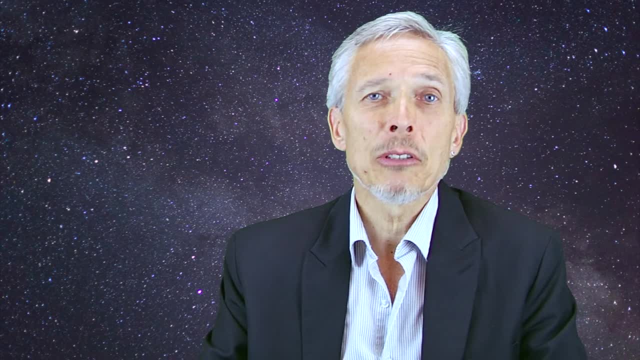 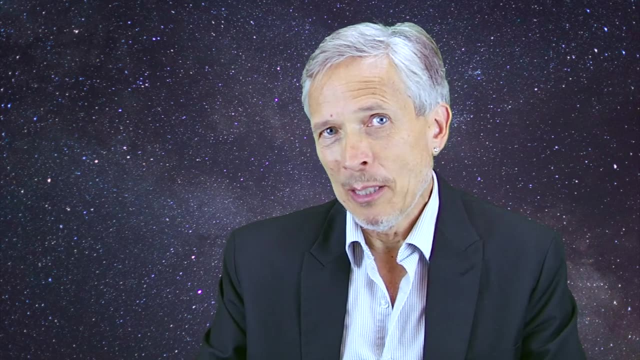 a phenomenon so remote from terrestrial experience. But let's use a terrestrial analogy. Imagine you're flying in a helicopter far above the city of Los Angeles at night. Now, there are not as many lights in Los Angeles streets and houses as there are stars in a galaxy. 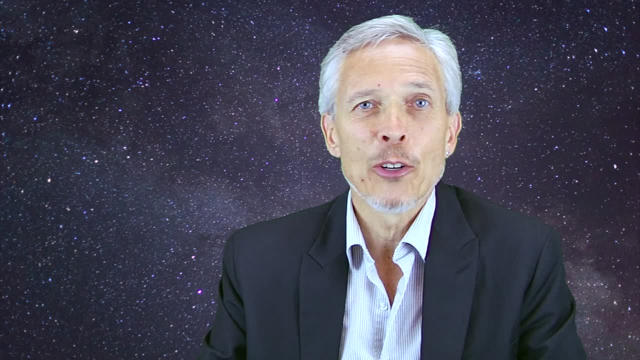 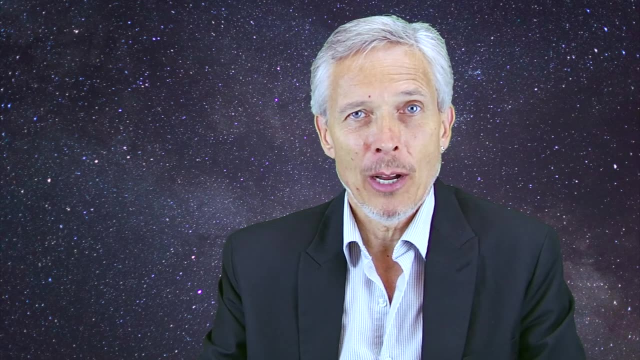 There's perhaps one light for every hundred stars in a galaxy, A hundred million lights maybe. Imagine those lights are stars and that Los Angeles is a gigantic galaxy that you're looking down upon. Imagine you go far above the Earth until the galaxy becomes small and difficult to see.